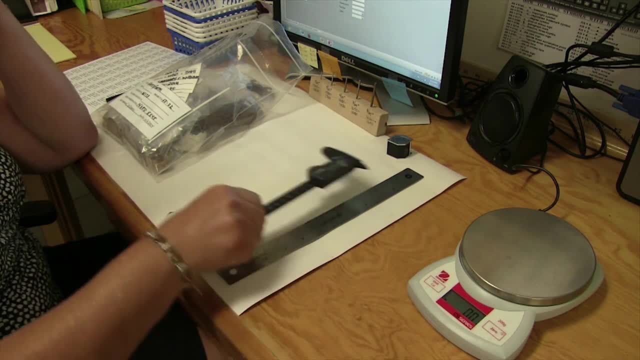 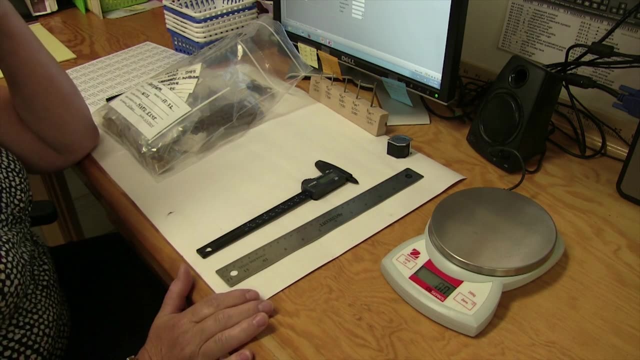 so we have a ruler and we have a different kind of ruler. We have a scale, One of the things we have a scale for, and then we have a ruler We- because we do measure besides measuring, we weigh everything. I also have this. 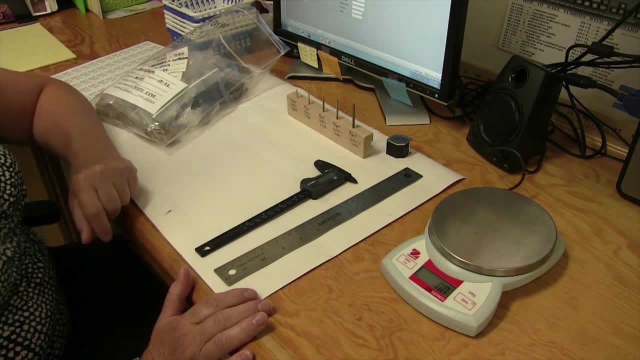 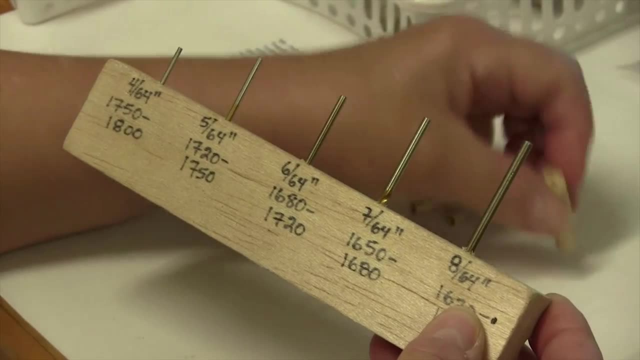 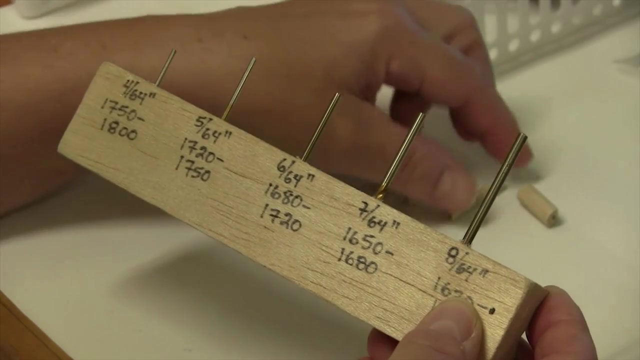 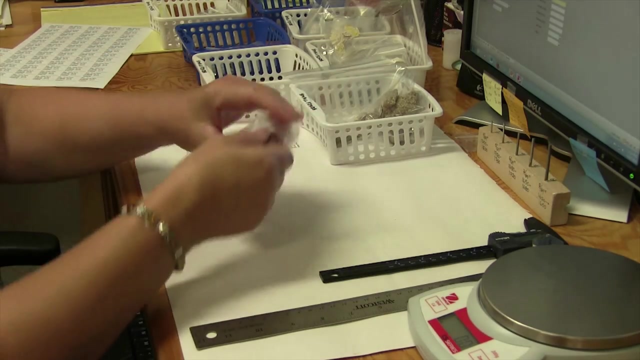 interesting little measuring tool. It measures the bores of pipe stems. According to how big the bore stem is, it corresponds roughly to an age and date. So the larger the diameter of the pipe stem, the earlier it is. So we're going to. 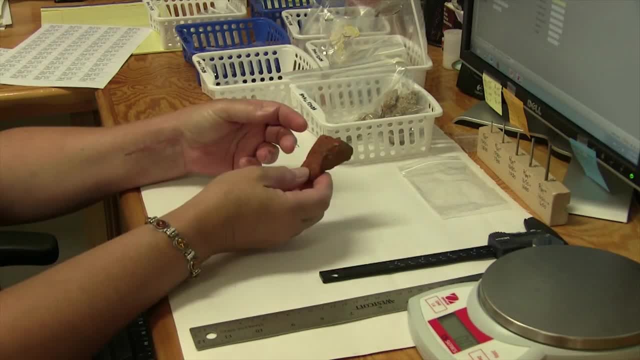 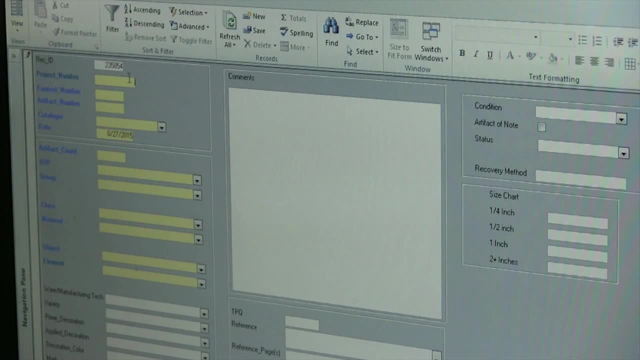 do the first artifact, and it happens to be a piece of brick, So the first. I'm going to describe this brick. in our database There's some beginning information that you have to put in. You have to put in the project number, which is FF22, the context number In this context. 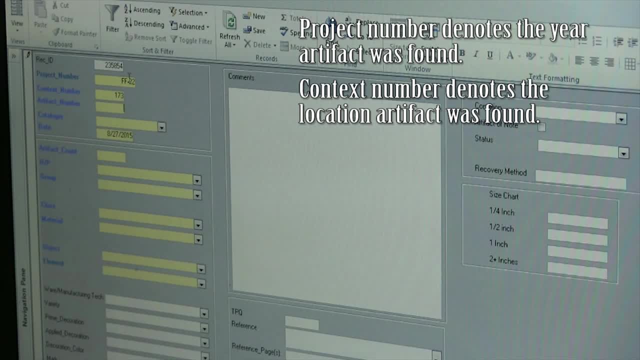 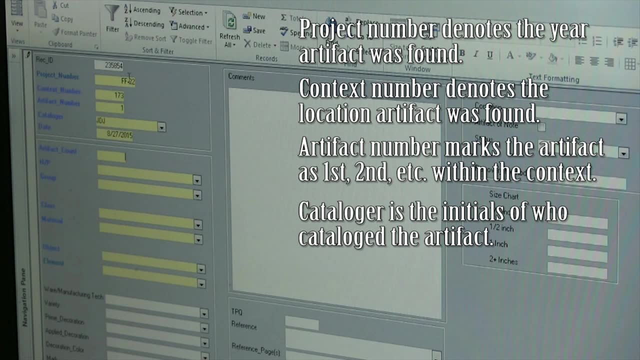 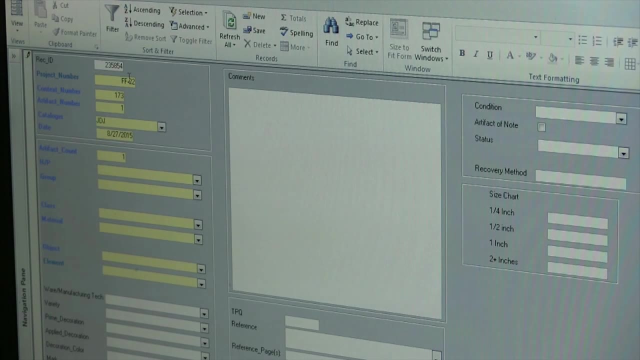 text number is 173. it is artifact number one. the cataloger is myself, so I put in my initials the artifact count. there's one brick, so I put in one, if there's two, I put in two, etc. etc. and then the next part is where I start describing the 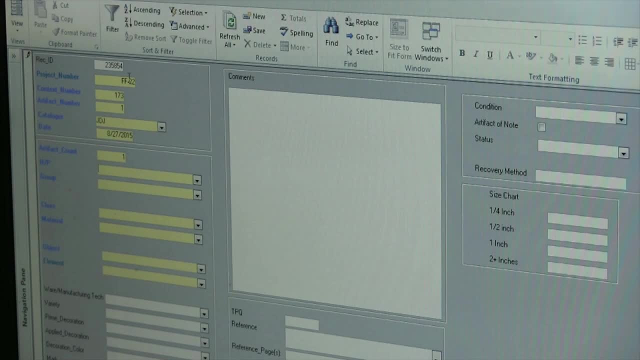 brick and the first category is: it is a historic artifact, it is an architectural element. the class indicates that it is ceramic and material is a courseware. the object is a brick. so type in brick: the element is a fragment. the manufacturing technique is that is handmade. I'm not going to measure this. 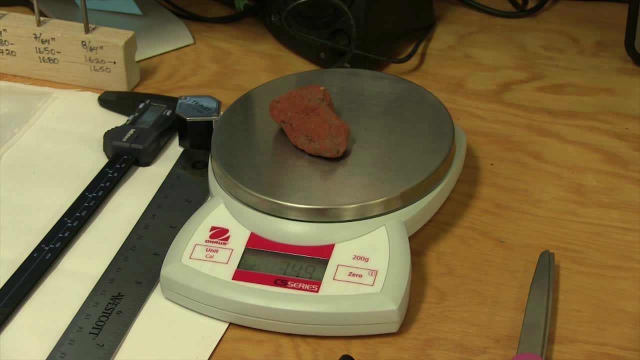 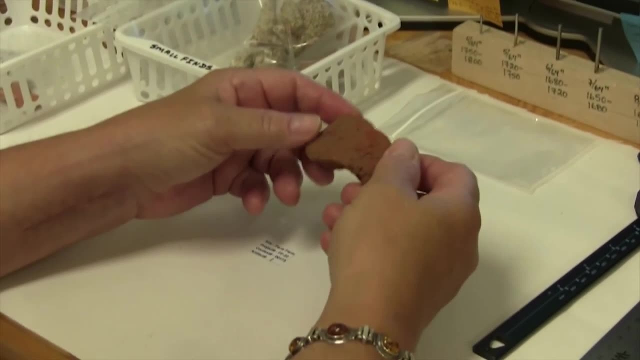 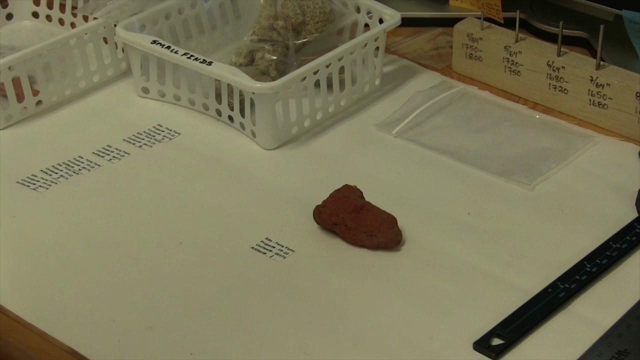 but I am going to weigh it: it is 30- 34.9 grams. If there was anything else about this brick that was distinctive, if it was burned or had some special inclusions, I could also put that information here in our database.